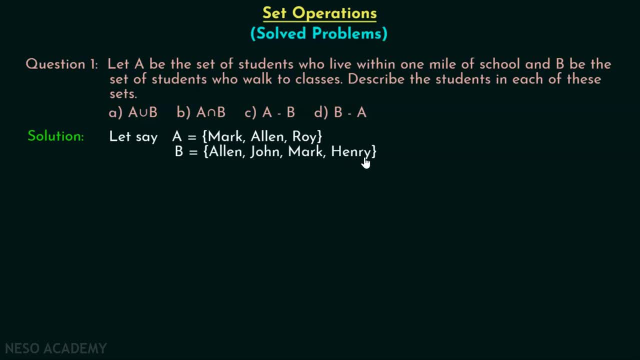 Okay, these are the elements of A and these are the elements of B. There are total three elements in A and four elements in B. A represents a set of all students who live within one mile of school and B represents a set of students who walk two classes. 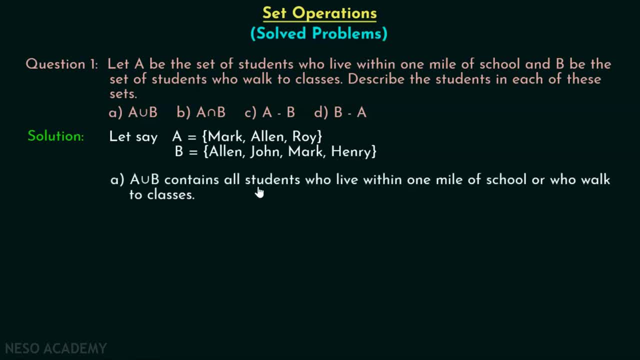 Okay, what is A union B? A union B contains all students who live within one mile of school or who walk two classes right, That means we must include all the students which are there in A and all students which are there in B. 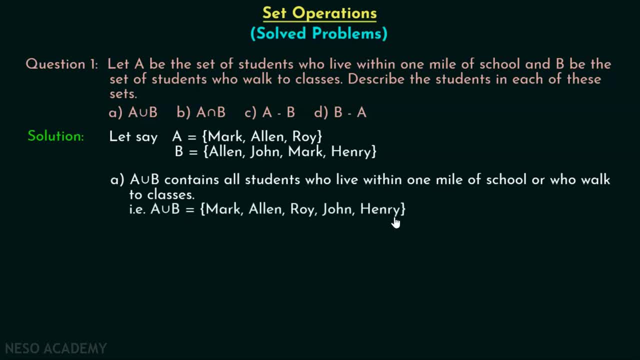 So A union B must be Mark, Alan, Roy, John Henry. That means all elements of A and all elements of B. In other words, we can say that we must include all students who live within one mile of school only, or who walk two classes or both. 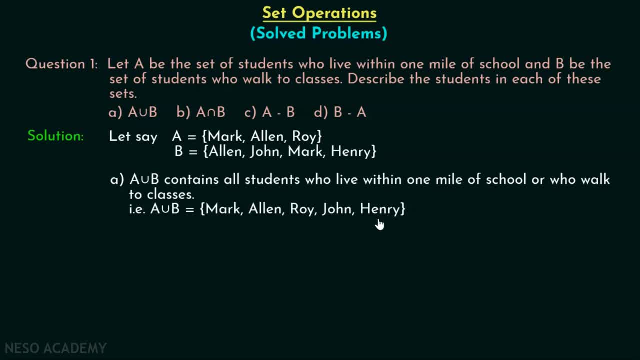 Okay, so Mark Alan Roy, John Henry, is the correct set. Now, what is A intersection B? A intersection B contains all students who live within one mile of school. All students who live within one mile of school and who walk two classes. 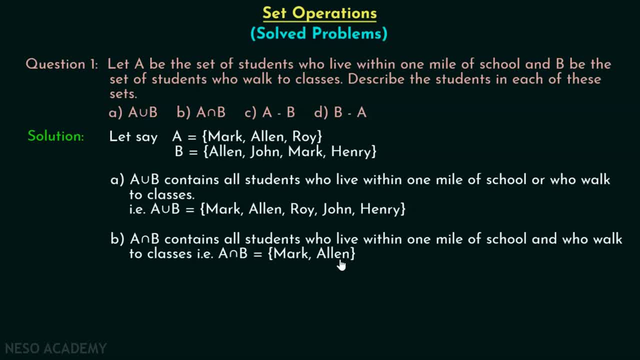 That is A intersection B must include Mark and Alan, right? We are talking about all students who live within one mile of school and who walk two classes. That means we are talking about common elements between A and B And we can see Mark and Alan is common between A and B. 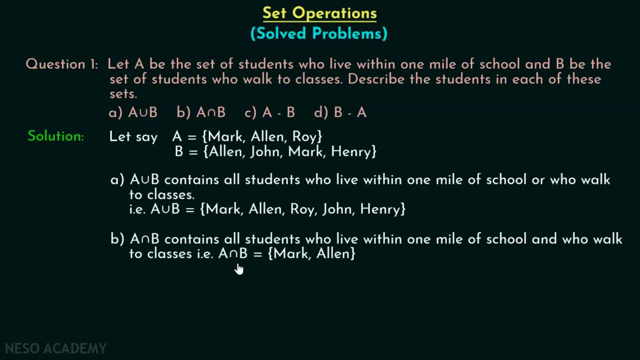 Thus Mark and Alan must be included in A intersection B. Now what is A minus B? A minus B contains all students who live within one mile of school but who do not walk two classes, right. right, That is A minus B must include Roy and nothing else. You can see that in set A and B. 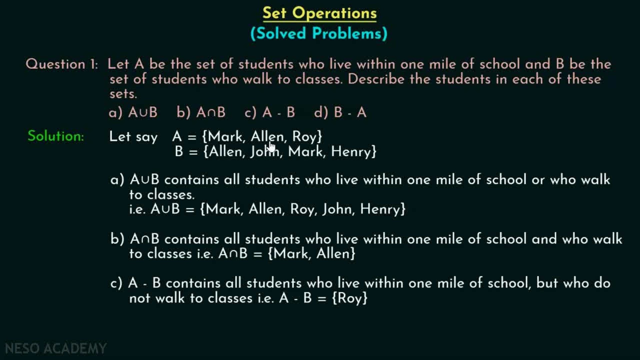 Mark and Alan are common elements. right, We have Mark Alan here and in set B also, we have Mark Alan. So Roy must be included in A minus B. Now, what is B minus A? B minus A contains all students who walk to classes but do not live within one mile of school. That is, B minus A must include. 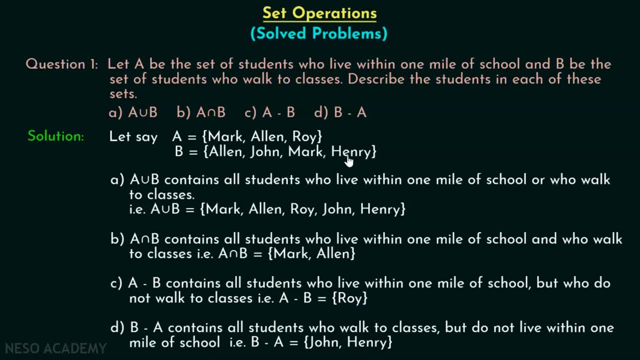 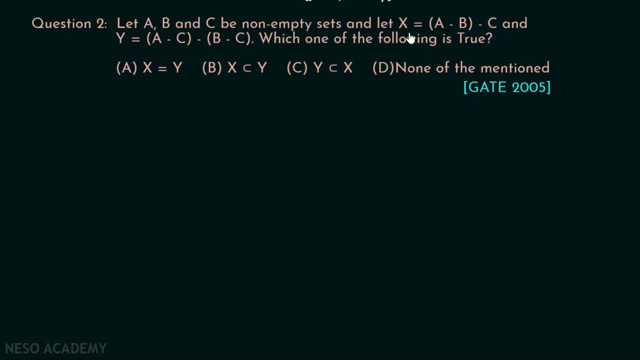 John Henry. You can see John Henry is there in set B, but it is not there in set A. So it is clear that B minus A must include John Henry, Isn't that? so Now let's discuss question number two. So here is question number two. Let A, B and C be non-empty sets and let X represents this. 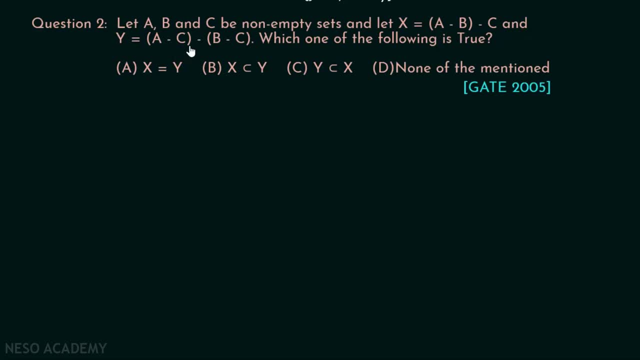 A minus B minus C and Y represents A minus C minus B minus C. Which one of the following is true? We have to answer this. which of the following option is true? This question has been asked in GATE 2005.. Let's just try to find the solution to this question. okay, We can find. 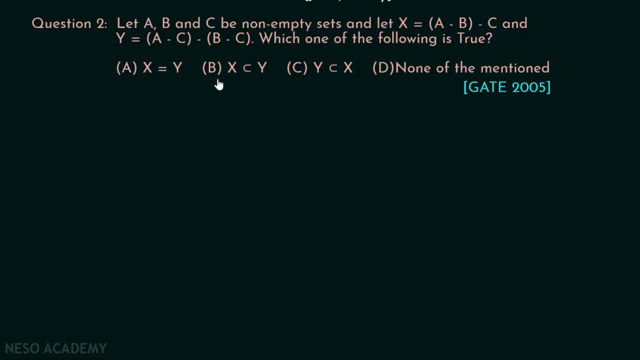 the solution to this question with different methods, but in my opinion, the best method is representing X and Y using Venn diagrams. okay, So here is how A minus B looks like, because in X we have A minus B minus C. Let's just first represent A minus B, and this is how it looks like. A minus B means only A and 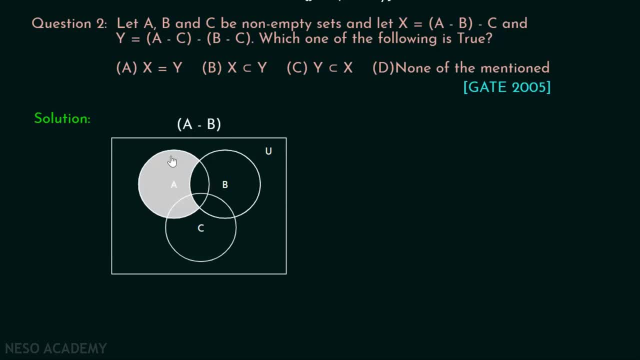 not B, right A but not B. This is how it looks like. Only A and not B. okay, There is nothing told about C. We should not consider C as a non-empty set. Let's just try to find the solution. 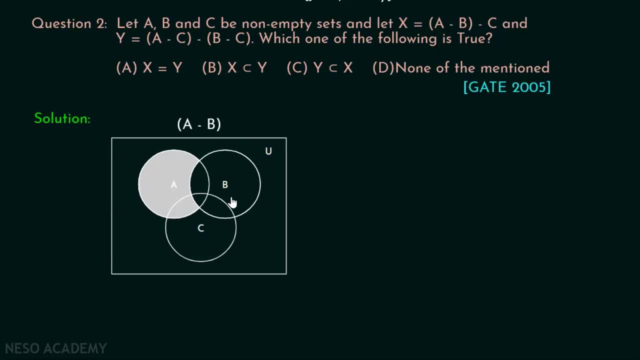 to this question. So if we are talking about C right now, we should only consider A and B sets. okay, And here you can see in this Venn diagram we have three overlapping circles, because here we are talking about three sets: A, B and C. So Venn diagram must have three overlapping circles. This 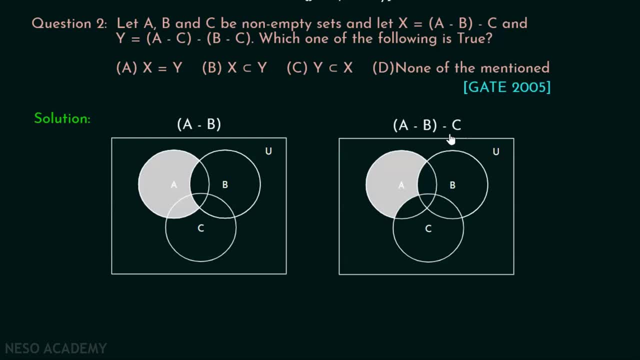 is A and not B. What is A minus B minus C? A minus B minus C must include only A minus B and not C. That means this overlapping region must not be included. okay, So after excluding this, we will get this particular set. 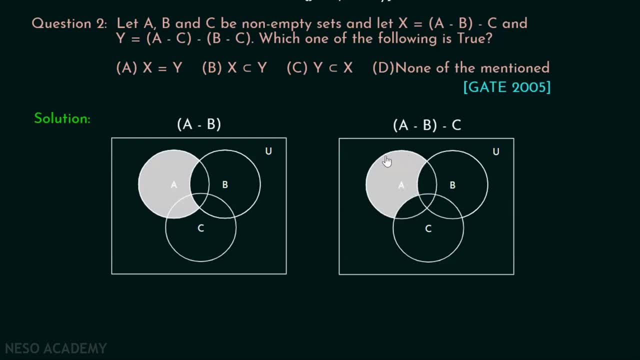 particular representation, Isn't that so? Here, this is the shaded region which represents a minus b minus c. Now let's see how to represent y, that is, a minus c minus b minus c, using Venn diagram. This is how a minus c looks like. 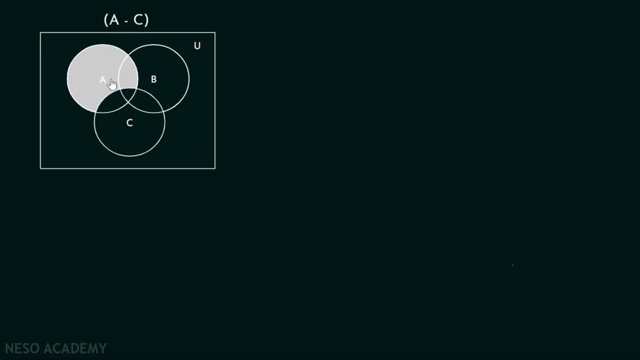 Here we have all a but not c, right. Only a and not c. And this is how b minus c looks like: Only b and not c, right? What is a minus c minus b minus c? This means we are only including a minus. 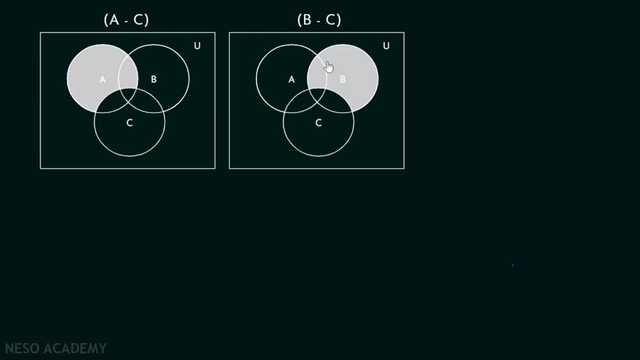 c and not b minus c. You can see this is the common portion between these two, So we should eliminate this, right? So this is how it looks like a minus c minus b minus c is nothing but this shaded region. right Now it is. 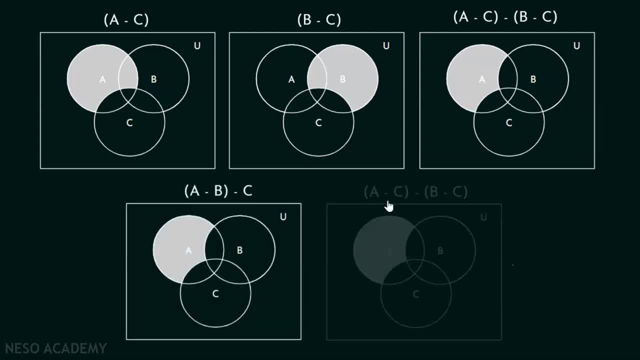 clear that a minus b minus c is actually equal to a minus c minus b minus c. You can see this pictorially right Through Venn diagrams. it is easier to visualize That a minus b minus c is actually equal to a minus. 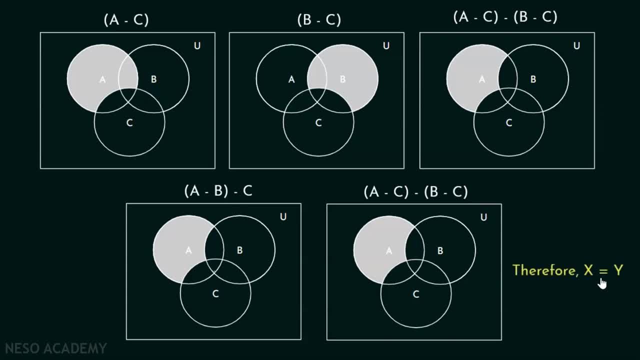 c minus b minus c. Therefore, we can say that x is equal to y. Now I want to discuss one alternative way of finding the solution to this question. Let's see the alternative way as well. This is the alternative way Here. 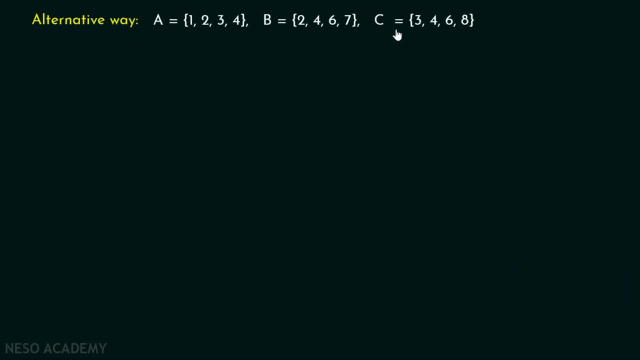 let's say that a represents this set, b represents this set and c represents this set. There are four elements each in these sets. In a, we have 1,, 2,, 3, 4.. In b, we have 2,, 4,, 6,. 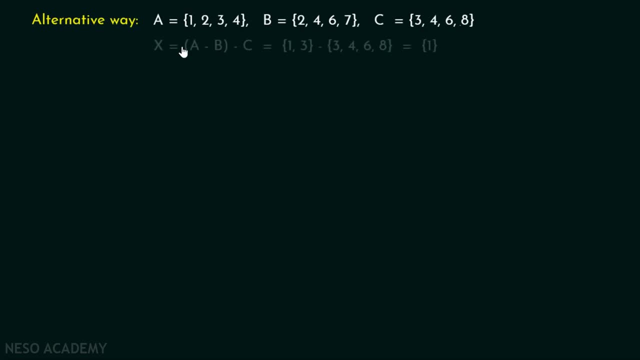 7 and in c we have 3,, 4,, 6,, 8.. Now, what is x? We know that x represents this: a minus b minus c. right? What is a minus b? Only a and not b. 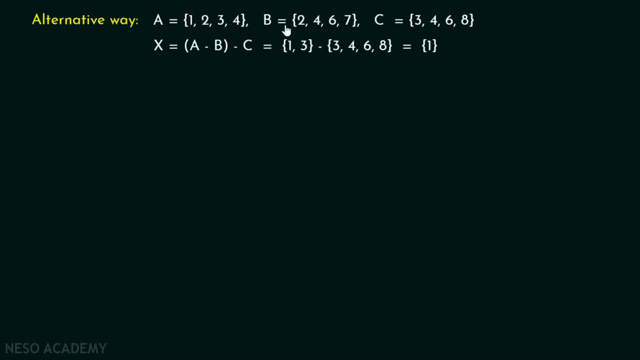 We can see that 2 and 4 is common in both these sets, So we should not include this in a minus b. We can only include 1 and 3.. That's why a minus b must be 1 comma 3.. Now 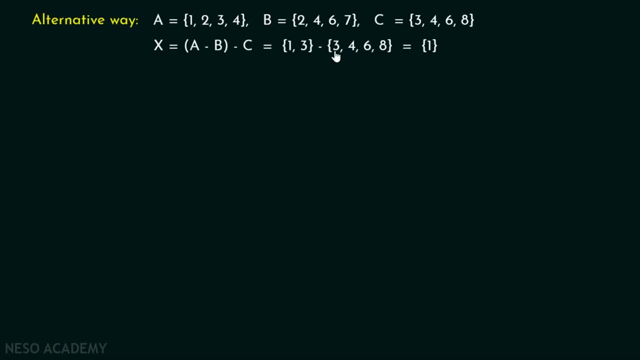 what is c? We know that c is 3,, 4,, 6, 8.. So let me just write this down over here. Now we have to find out what is the difference between these two sets. We can see that the difference between: 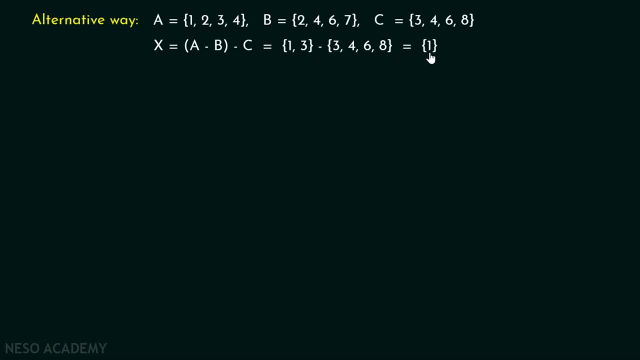 these two sets must be this set, which consists of just one element, and that is 1.. Because here you can see, in these two sets 3 is common and we must include all the elements of this set in the difference of these two sets. Therefore, 1 must 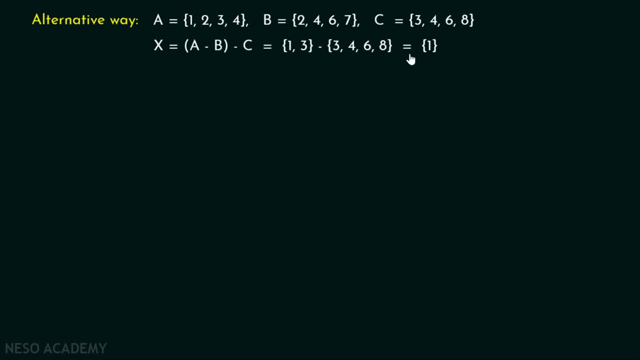 be included in the resultant set right. So x is nothing but this set, which consists of this element: 1.. And what is y? We know that y is equal to a minus c minus b minus c. right, What is a minus? 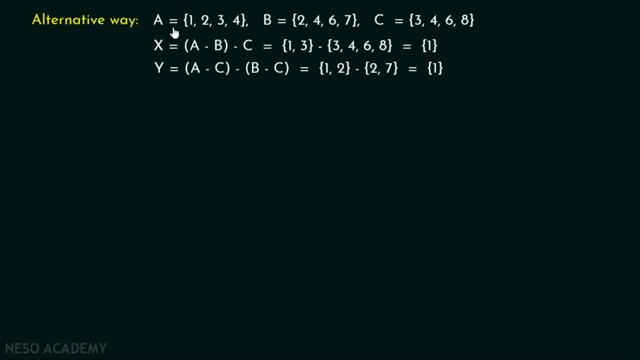 c. a minus c must include only a and not c, right? We can see that 3, 4 is common in both these sets. Therefore, 1, 2 must be included in a minus c, right? So you can see. 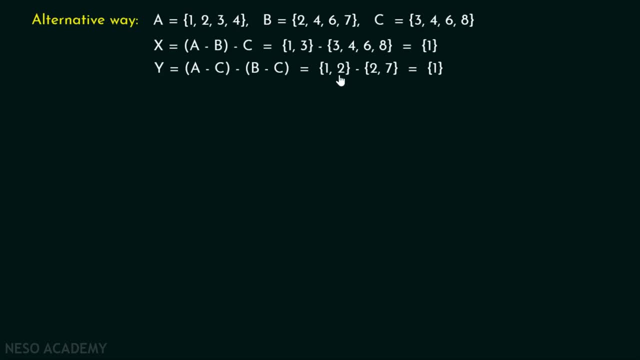 a set with these two elements: 1, 2.. This is a minus c. What is b minus c? b minus c must include elements that are there in b and not in c. You can see that 4 and 6 is common in these two sets.